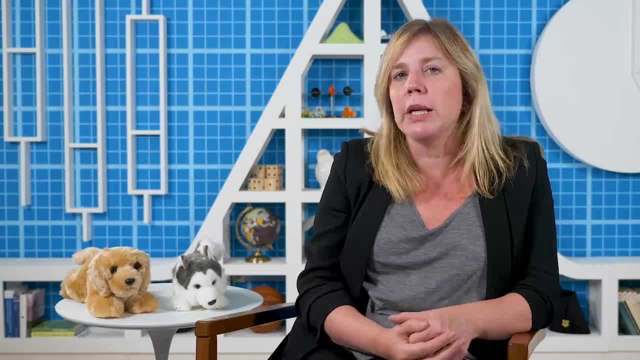 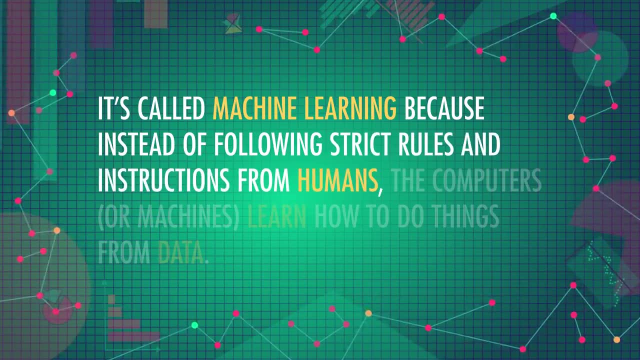 and tries to learn how to predict it. It's supervised because we can tell the model what it got wrong. It's called machine learning because, instead of following strict rules and instructions from humans, the computers or machines learn how to do things from data. 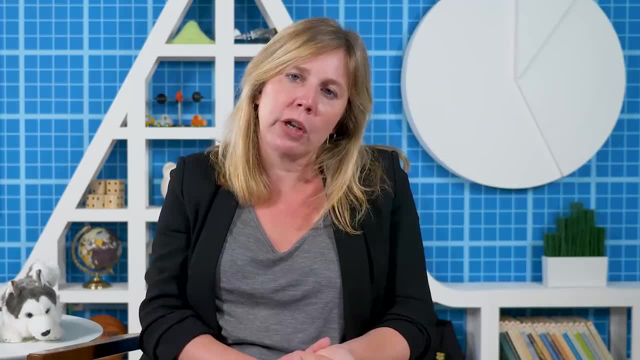 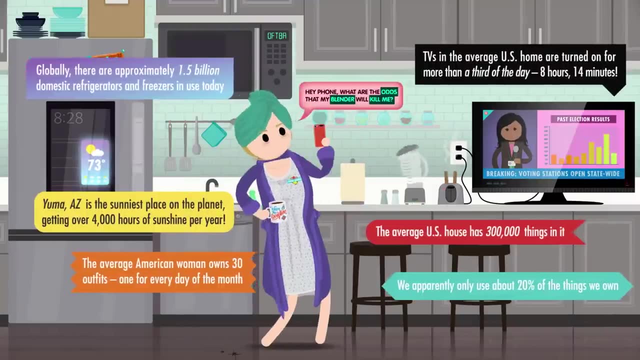 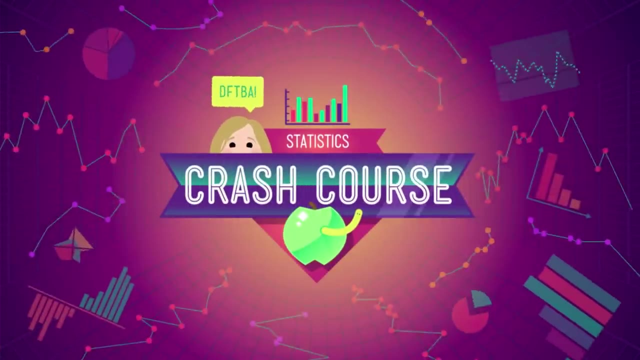 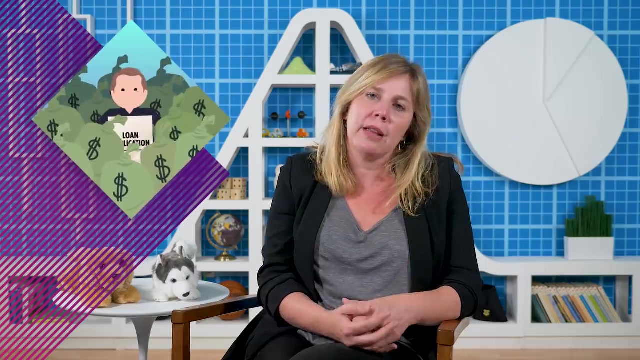 Today we'll briefly cover a few types of supervised machine learning models: Logistic regression, linear discriminant analysis and. k-nearest neighbors Say you own a microloan company. Your goal is to give short-term, low-interest loans to people around the world so they can invest in their small businesses. 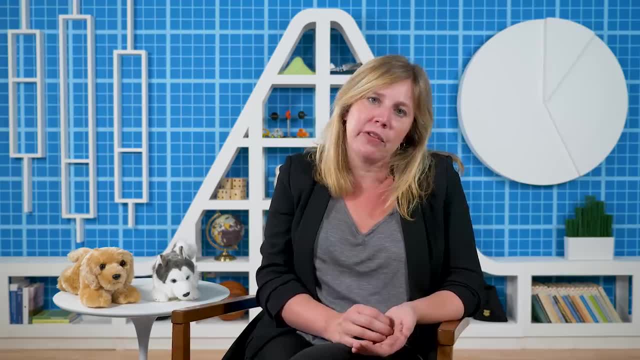 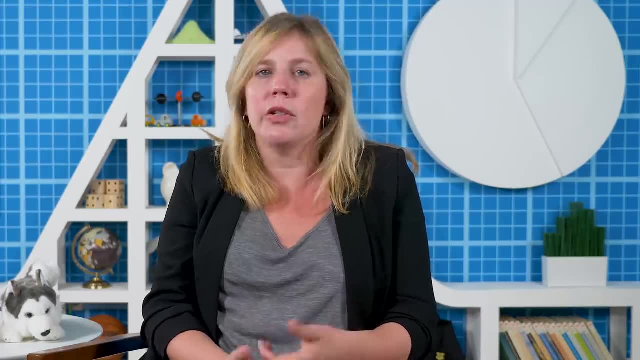 You have everyone fill out an application that asks them to specify things like their age, sex, annual income and the number of years they've been in business. The microloan is not a donation. The recipient is supposed to pay it back, so you need to figure out who is most likely. 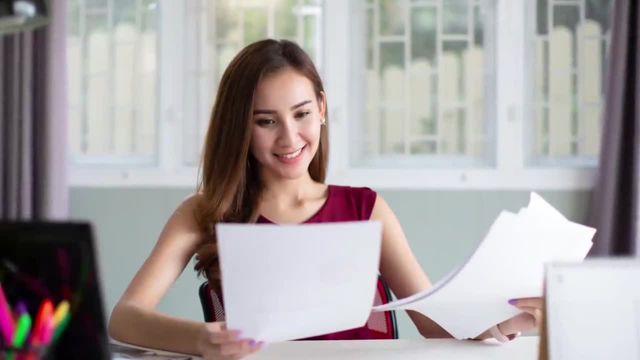 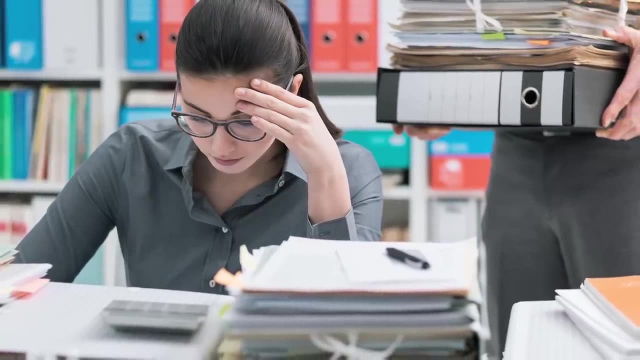 to do that. During the early days of your company, you reviewed each application by hand and made that decision based on personal experience of who was likely to pay back the loan. But now you have more money, men and women. You have more money than applicants, than you could possibly handle. 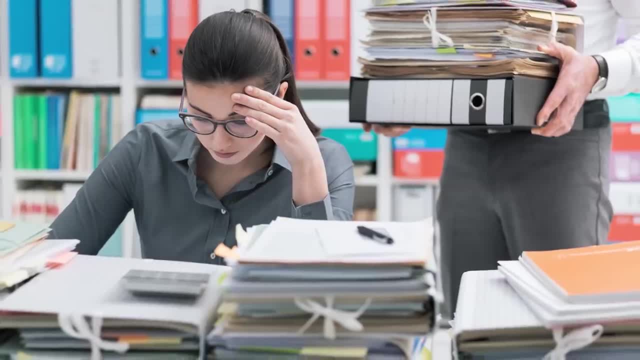 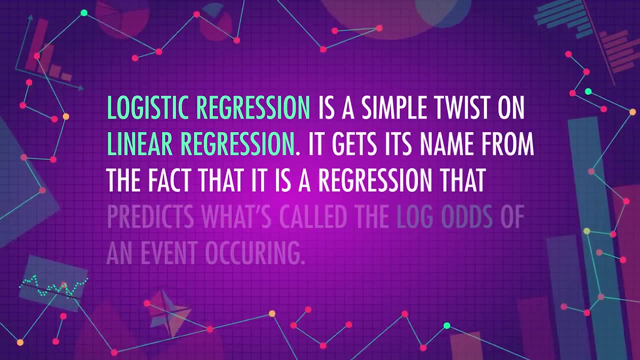 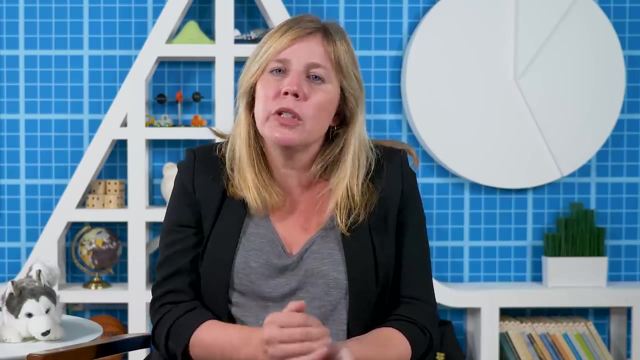 You need a model or algorithm to help you make these decisions efficiently. Logistic regression is a simple twist on linear regression. It gets its name from the fact that it is a regression that predicts what's called the log odds of an event occurring. While log odds can be difficult, once we have them we can use some quick calculations to 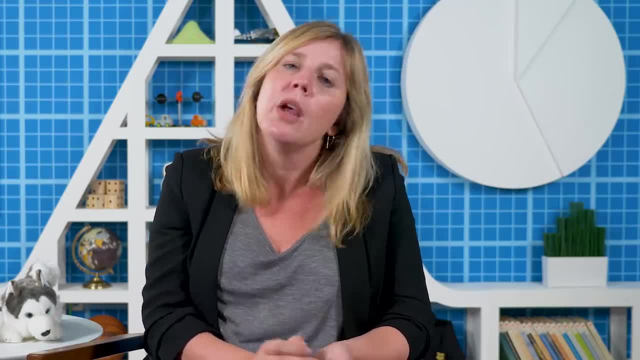 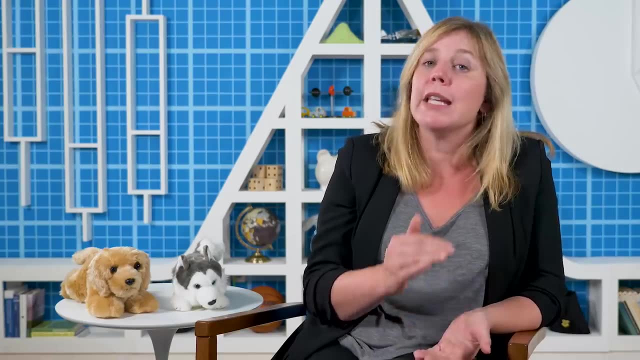 turn them into probabilities which are a lot easier to work with. We can use these probabilities to predict whether an individual will default on their loan. Usually, the cutoff is 50%. If someone is less than 50% likely to default on their loan, we'll predict that they'll. 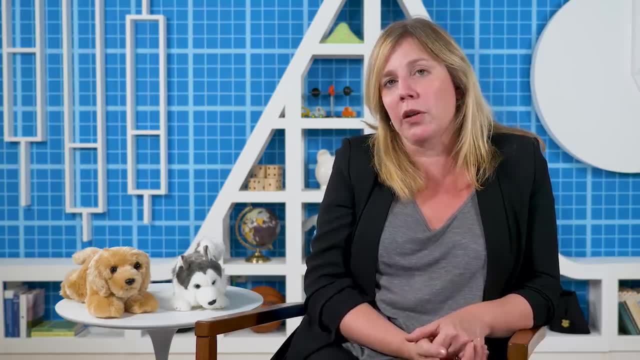 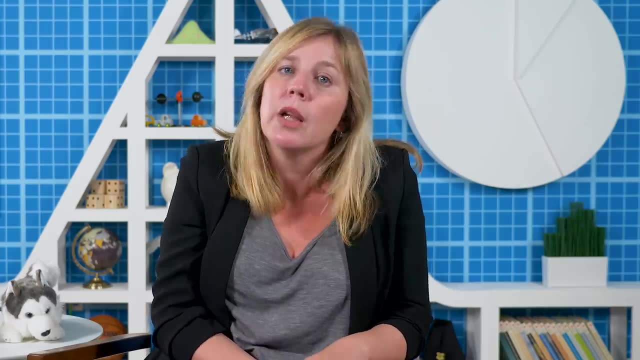 pay it off. Otherwise, we'll predict that they won't pay off their loan. We need to be able to test whether our model will be good at predicting data it's never seen before data it doesn't have the correct answer for, So we need to pretend that some of our data is future data for which we don't know. 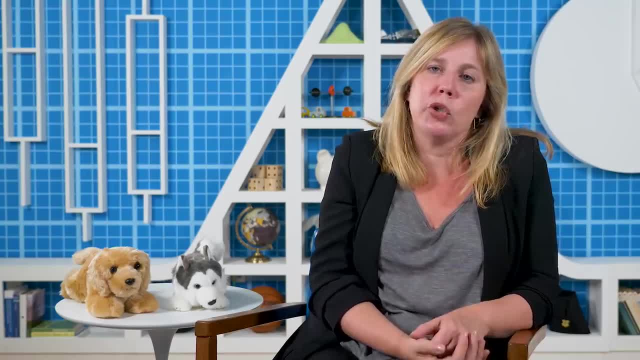 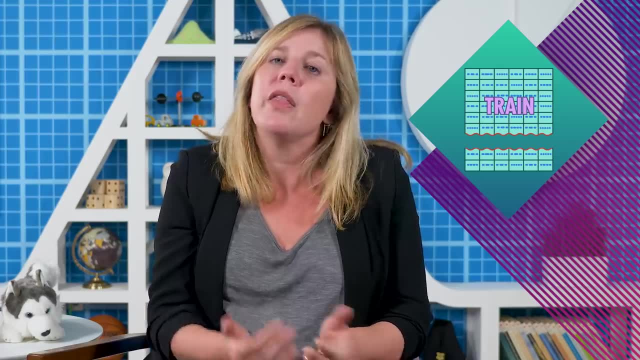 the outcome. One simple way to do this is split our data into two parts. The first portion of our data, called the training set, will be the data we use to create or train our model. The other portion, called the testing set, is the data we're pretending is from the 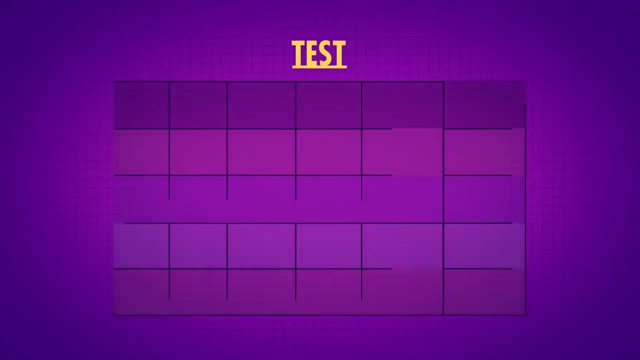 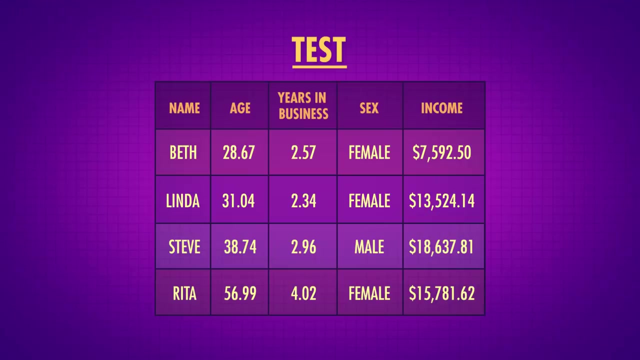 future. We don't use it to train our model, Instead to test how well our model works. we withhold the outcomes of the test set, So the model doesn't know whether someone paid off their loan or not, and we ask it to make a prediction. 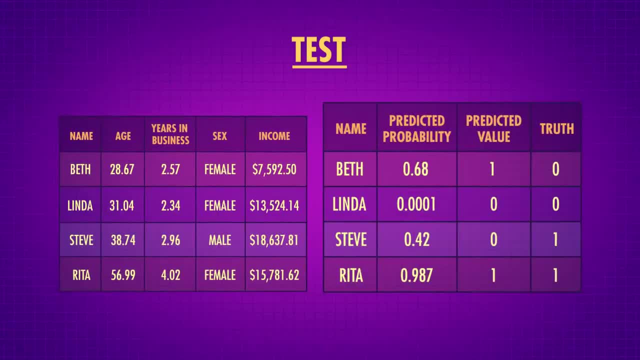 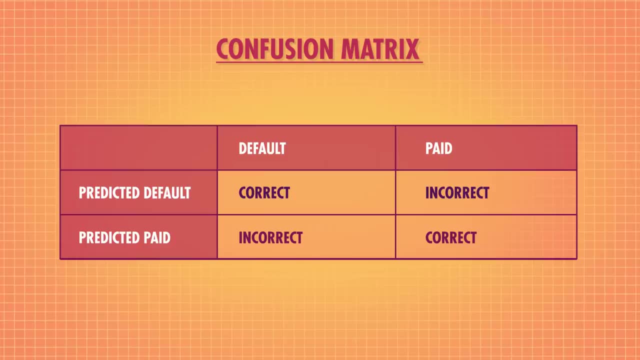 Then we can compare these with the real outcomes that we ignored before. We can do this using what's called a confusion matrix. A confusion matrix is a chart that tells us what happens when a person defaults on their loan. It tells us what actually happened, whether a person paid back a loan and what the model. 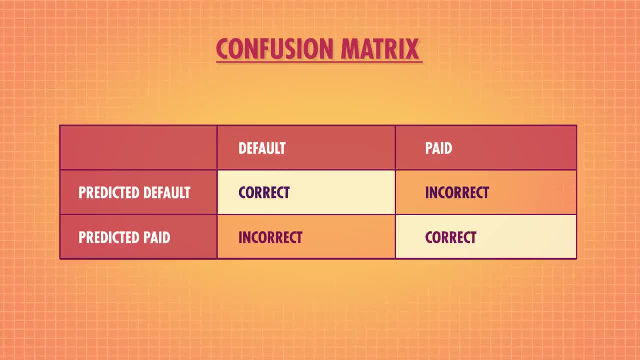 predicted would happen. The diagonals of this matrix are the times when the model got it right. Cases where the model correctly predicted that the person will default on the loan is called a true positive. true because it got it right, positive because the person defaulted. 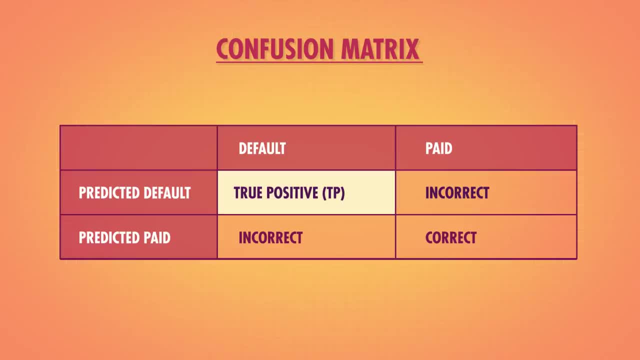 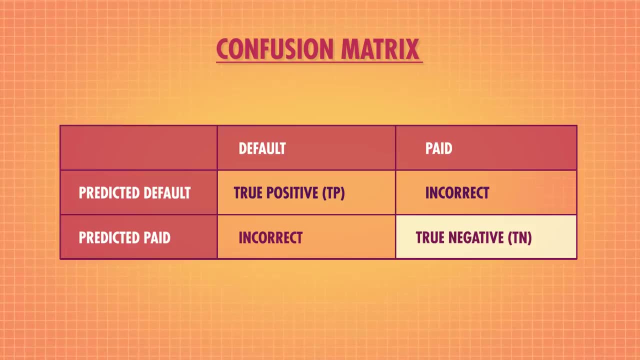 on their loan. Cases where the model correctly predicted that a person will pay back the loan are called true negatives- again: true because it made the correct prediction and negative because the person didn't default. Cases where the model was wrong are called false negatives- if the model thought they. 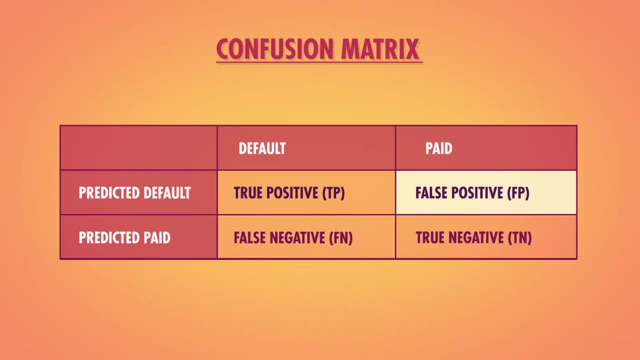 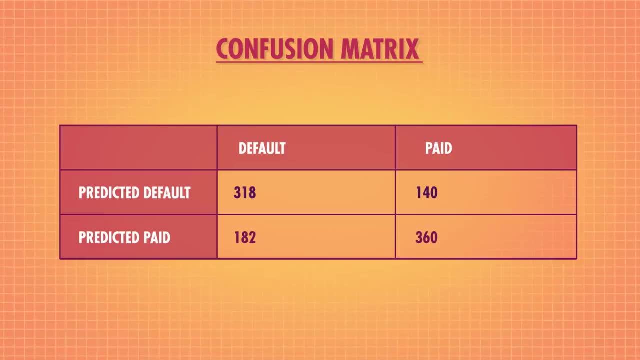 would not default and false positives if the model thought they would default. Using current data and pretending it was future data allows us to see how this model performed with data it had never seen before. One simple way to measure how well the model did is to calculate its accuracy. 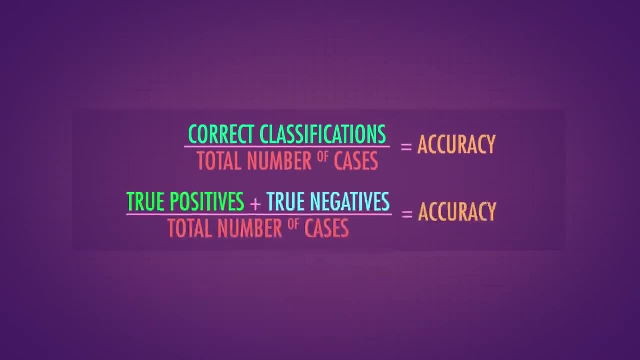 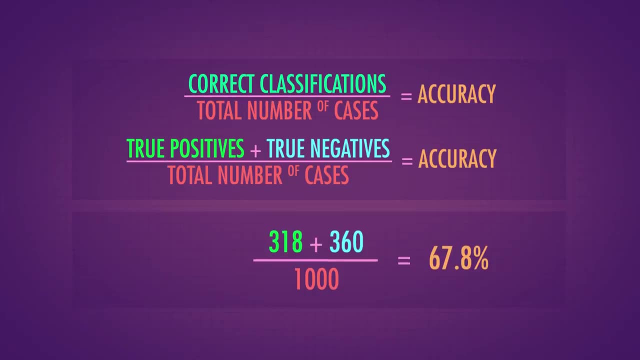 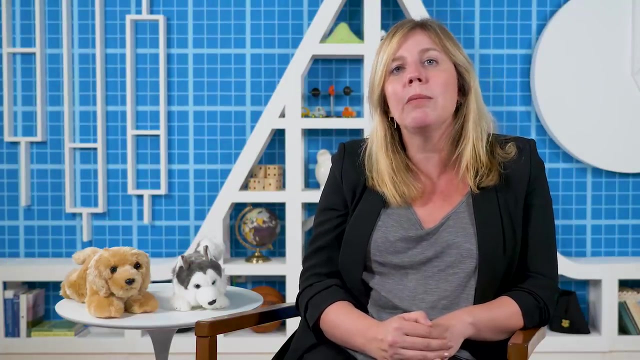 Accuracy is the total number of correct classifications, or true positives and true negatives, divided by the total number of cases. It's the percent of cases our model got correct. Accuracy is important, but it's also pretty simplistic. It doesn't take into account the fact that in different situations we might care more. 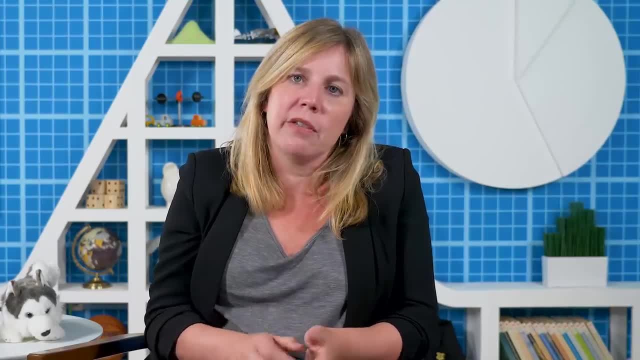 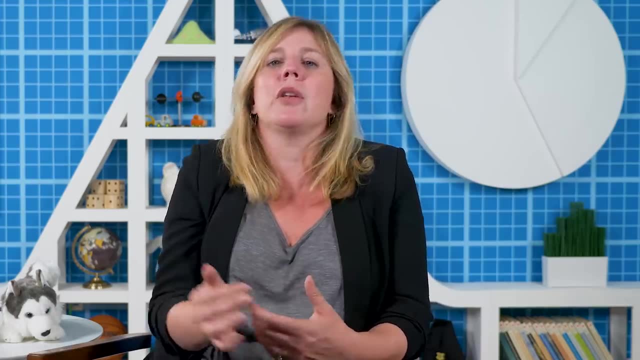 about some mistakes than others. We're not going to touch on other methods of measuring a model's accuracy here, But it's important to recognize that in many situations we want information above and beyond just an accuracy percentage. Logistic regression isn't the only way to predict the future. 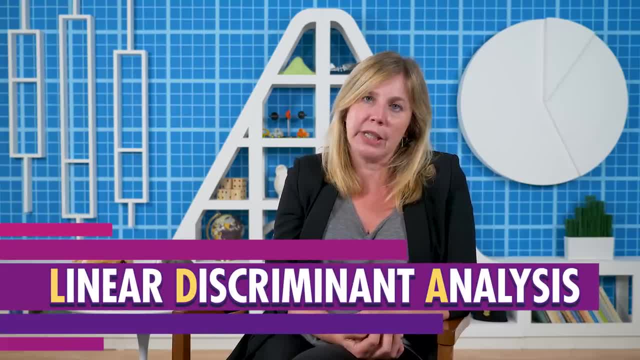 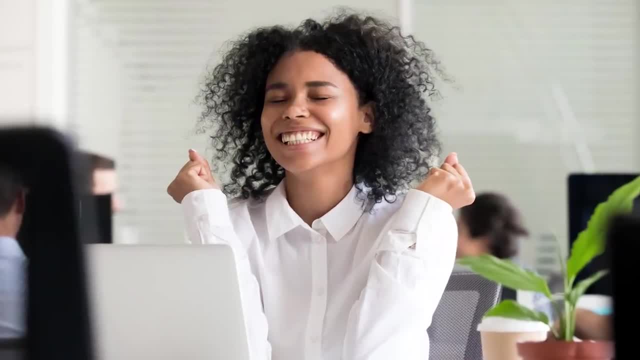 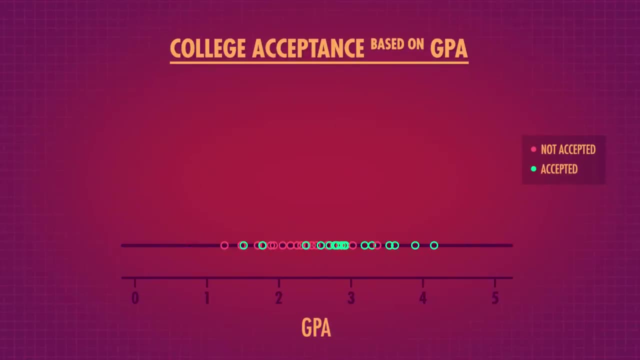 Another common model is linear discriminant analysis. LDA uses Bayes' theorem in order to help us make predictions about data. Let's say we want to predict whether someone would get into a local state college based on their high school GPA. The red dots represent people who did not get in, greener people who did. 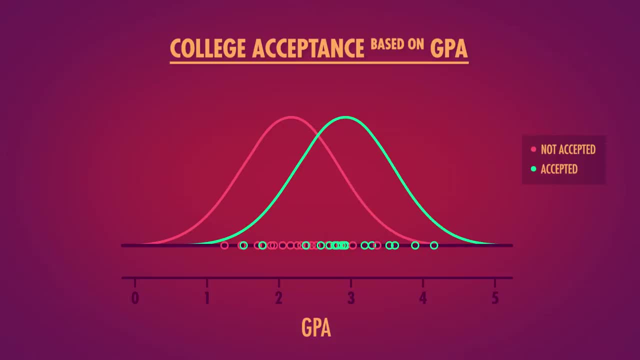 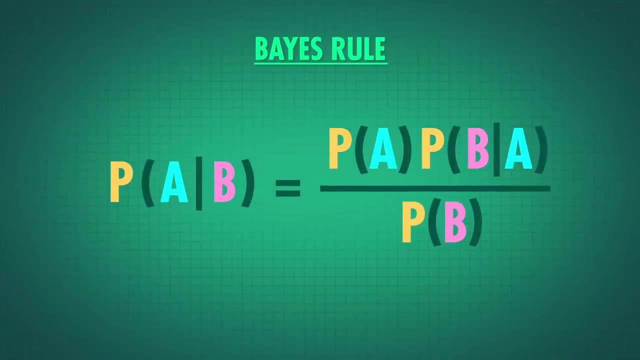 If we make a couple of assumptions, we can estimate the GPA distributions of people who did and did not get their acceptance letter. If we find a new student who wants to know if they will get into the college, we use Bayes' rule and these distributions to calculate the probability. 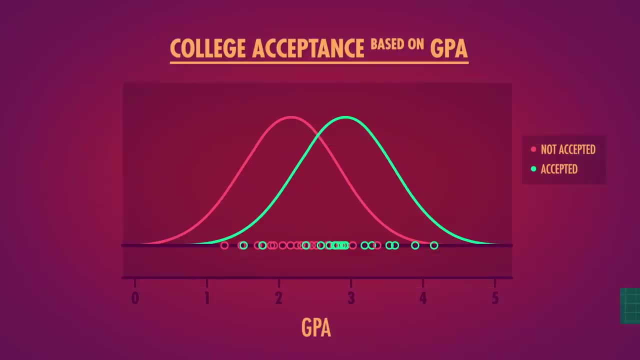 LDA just asks which category is more likely If we draw a vertical line at their GPA, whichever distribution has a higher value at that line is the group, we'd guess. Since this student, Annalisa, has a 3.2 GPA, we'd predict that she does get in, since 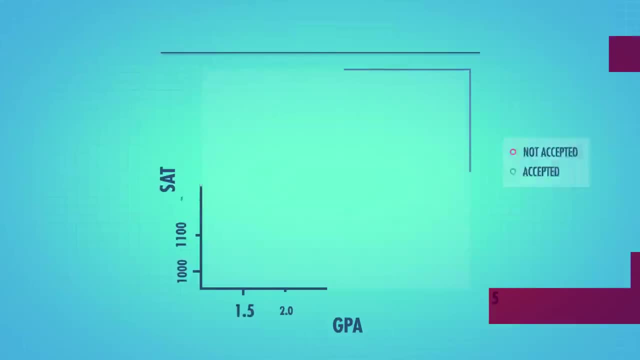 it's more likely under the got-in distribution. But we all know that GPA isn't everything. What if we looked at SAT scores as well? Looking at the distributions of both GPA and SAT scores, we can see that the GPA distribution is higher than the GPA distribution. 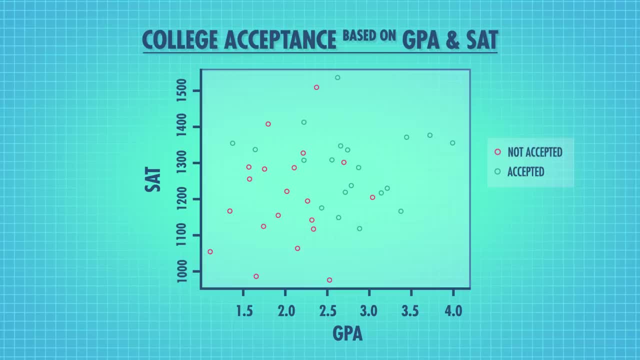 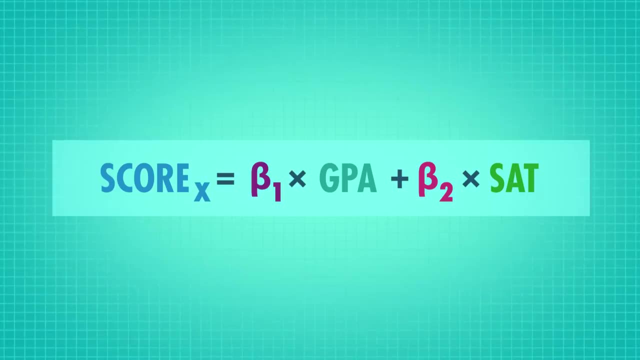 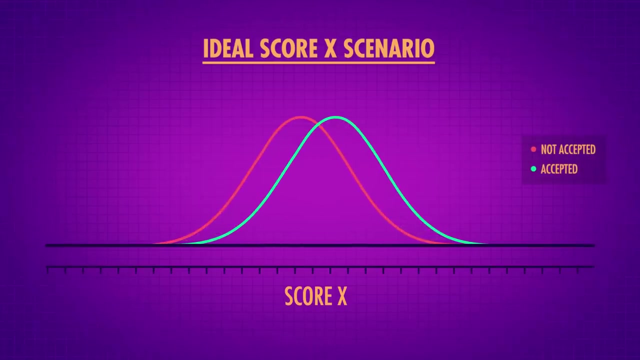 The GPA distribution is higher than the GPA distribution. This is where LDA becomes really helpful. We want to create a score- We'll call it score X- that's a linear combination of GPA and SAT scores, Something like this. We, or rather the computer, want to make it so that the score X value of admitted students. 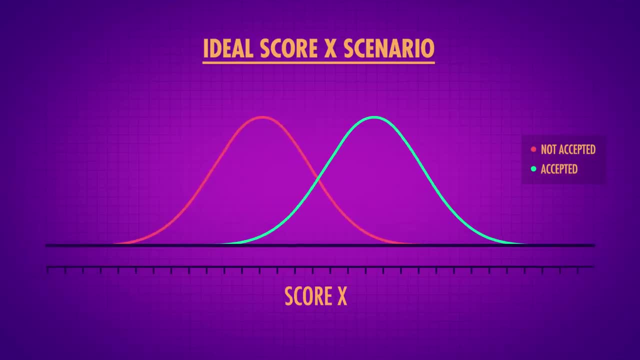 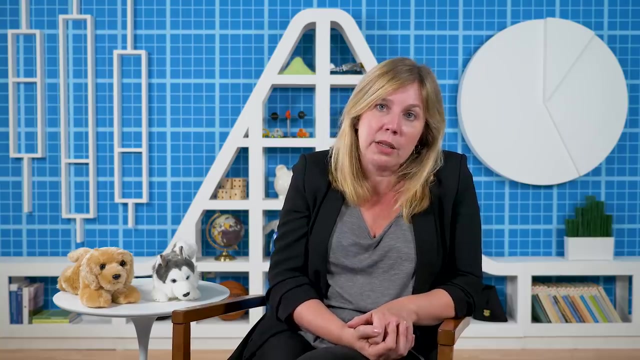 is as different as possible from the score X value of the people who weren't admitted. This special way of combining variables to make a score that maximally separates the two groups is what makes LDA really special, really special. So score X becomes a pretty good indicator of whether or not a student got in. 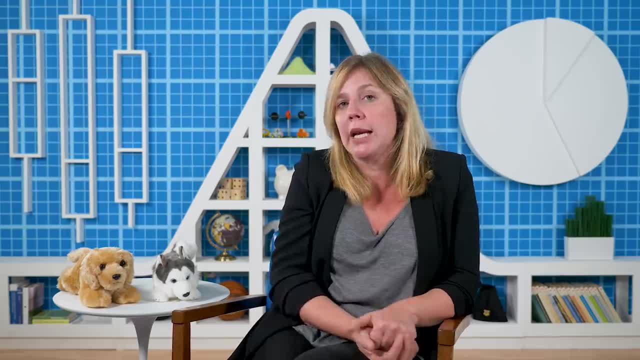 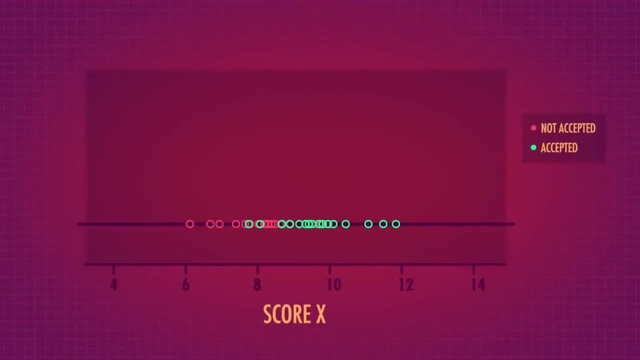 And it's one number that we have to keep track of. instead of two GPA and SAT score For this sample, my computer told me that this is the correct formula, Which means we can take the scatterplot of both GPA and SAT score and change it into. 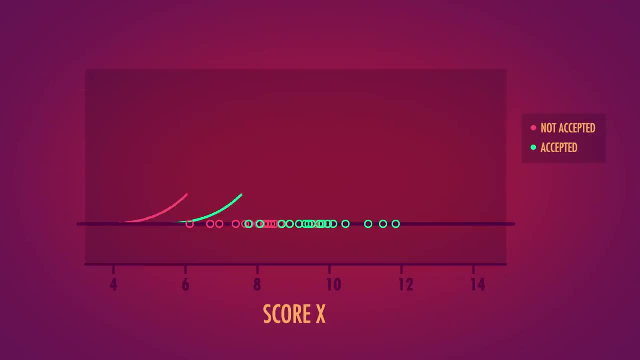 a one-dimensional graph of just score X. Then we can plot the distribution and use Bayes' rule to predict whether a new student, Brad, is going to get into the school. Brad's score X is 8, so we predict that he won't get in. 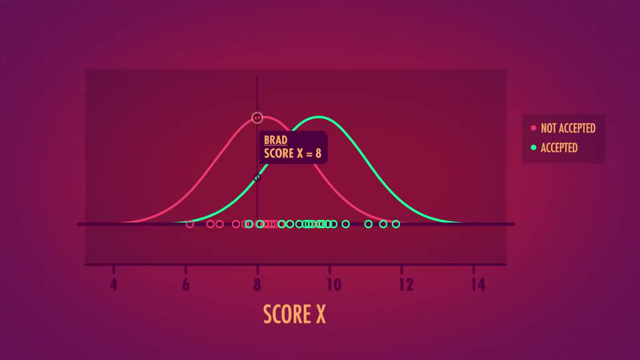 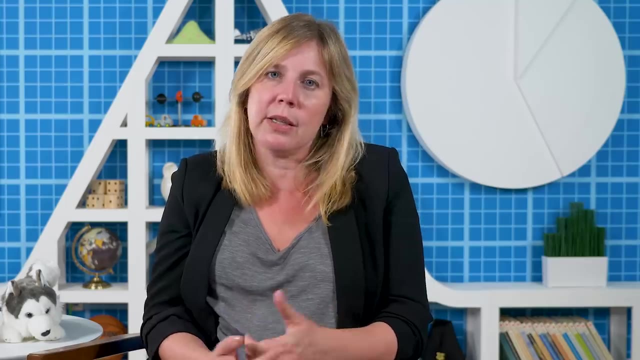 Since with a score X of 8, it's more likely that you won't get in than that you will. Creating a score X can simplify things a lot. Here we looked at two variables which we could have easily graphed, But that's not the case if we have 100 variables for each student. 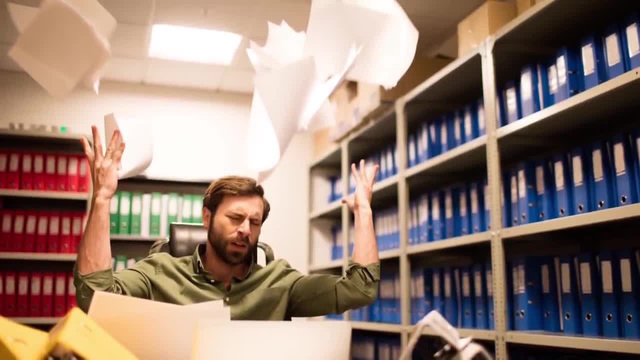 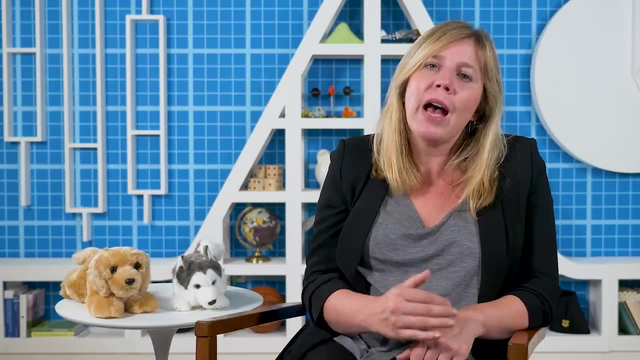 And, trust me, you don't want your college admissions counselor making admissions decisions on a graph like that. Using fewer numbers also means that on average, the computer can do faster calculations. So if 5 million potential students ask you to predict whether or not they get in using 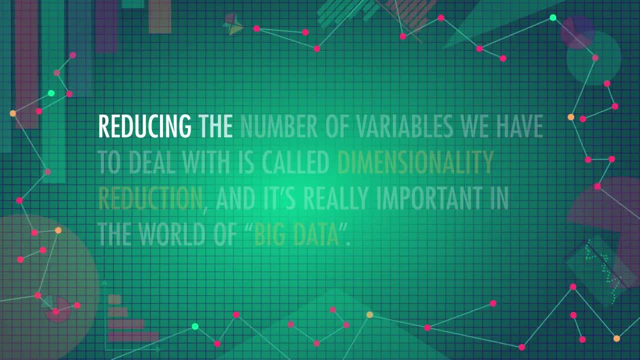 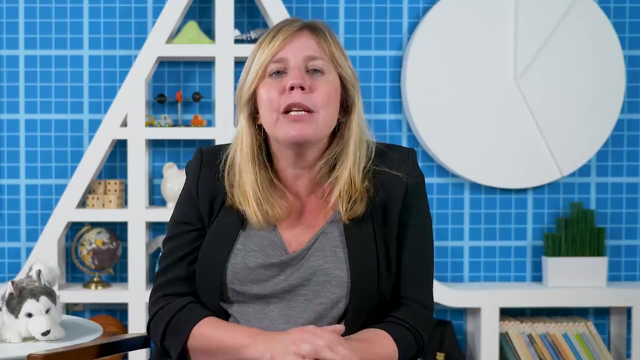 LDA, to simplify, will speed things up. Reducing the number of variables we have to deal with is called dimensionality reduction, And it's really important in the world of big data. It makes working with millions of data points, each with thousands of variables, possible. 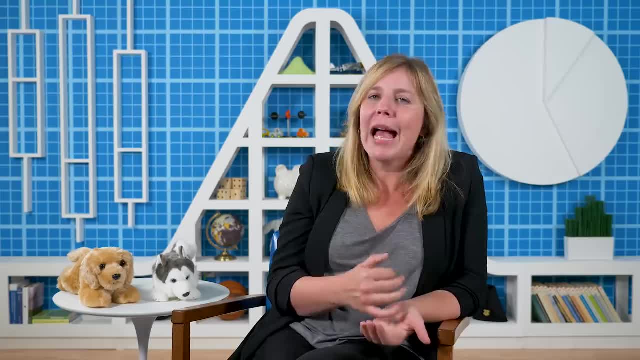 And that's often the kind of data that companies like Google and Amazon have. The last machine learning model we'll talk about is k-nearest neighbors. K-nearest neighbors, or KNN, relies on the idea that the number of variables that a student 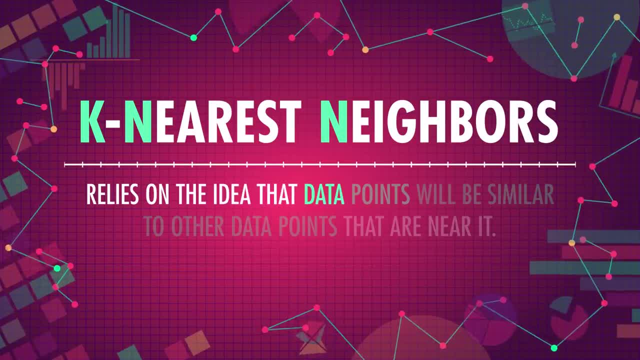 is able to get in is less than the number of variables that a student is able to get in. So if 5 million potential students ask you to predict whether or not they get in, using LDA to simplify, it makes sense, But it also gives us the idea that data points will be similar to other data points. that 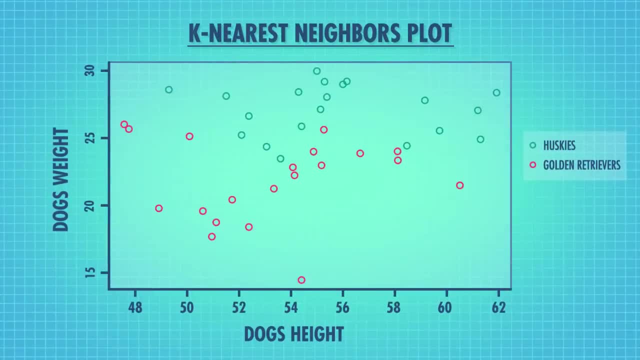 are near it. For example, let's plot the height and weight of a group of golden retrievers and a group of huskies. If someone tells us a height and weight for a dog named Chase, whose breed we don't know, we could plot it on our graph. 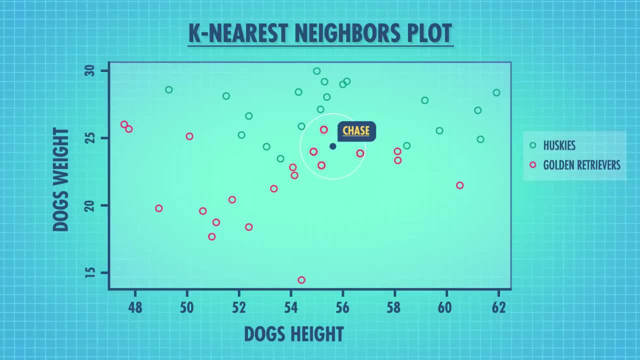 The four points closest to Chase are golden retrievers, so we could guess he's a golden retriever. That's the basic idea behind k-nearest neighbors, Whichever category- in this case dog breed- has more data points near our new data point. 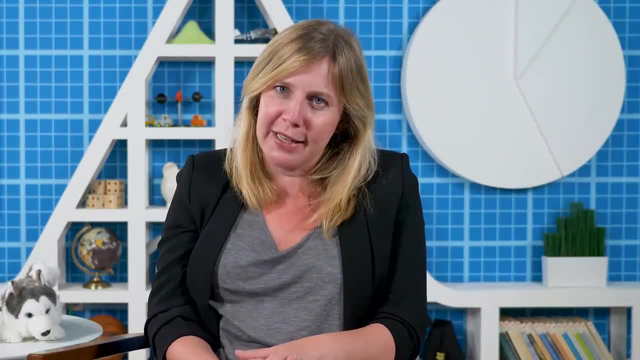 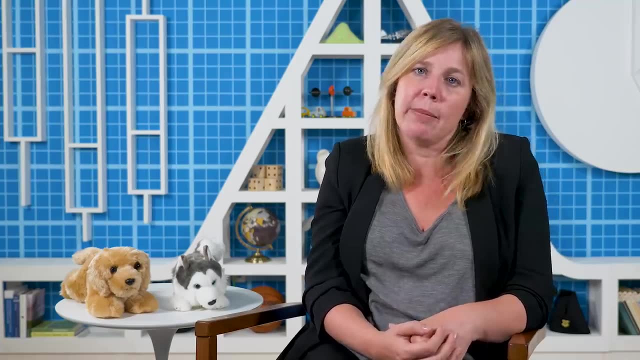 is the category we want. In practice, it's a tiny bit more complicated than that. One thing we need to decide is how many neighboring data points to look at. The k in k-n-n is a variable representing the number of neighbors we'll look at for. 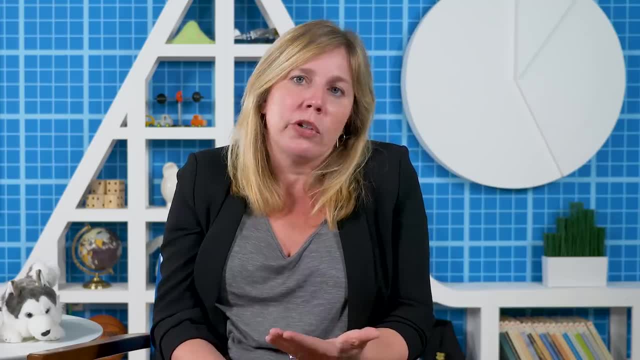 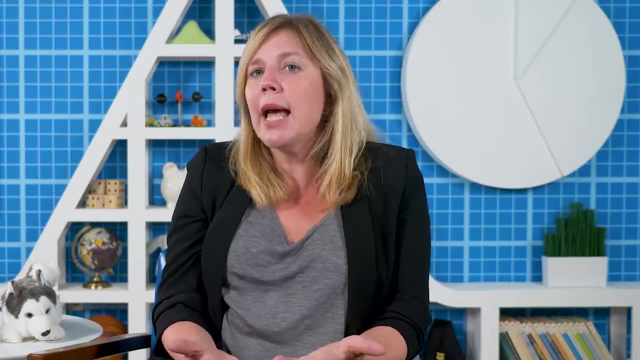 each point or dog we want to classify. When we wanted to know whether Chase was a husky or golden retriever, we looked at the four closest data points. so k equals 4.. But we can set k to be any number. 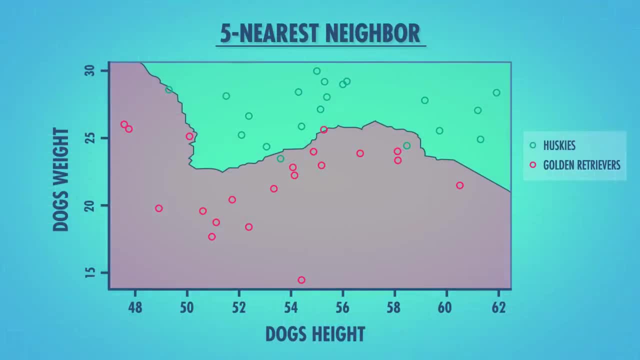 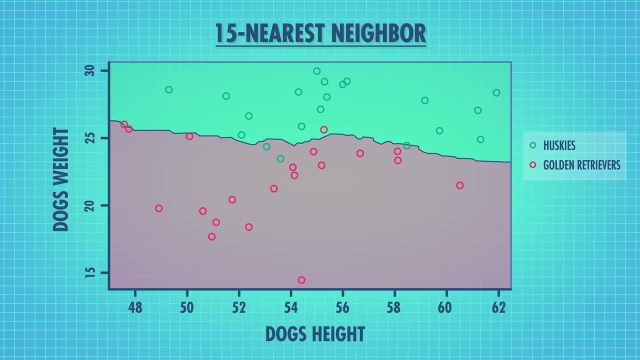 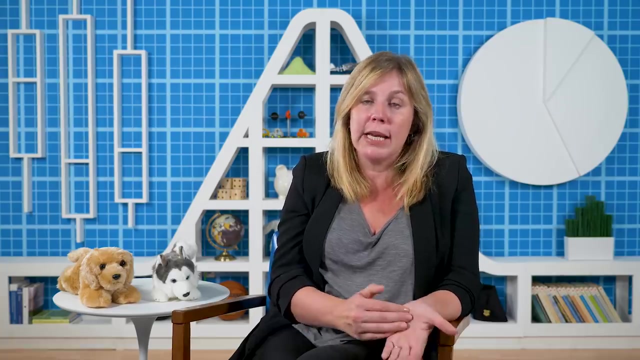 We could look at the one nearest neighbor or 15 nearest neighbors. as k changes are, classifications can change. These graphs show how points in each area of the graph would be classified. There are many ways to choose which k to use. One way is to split your data into two groups: a training set and a test set. 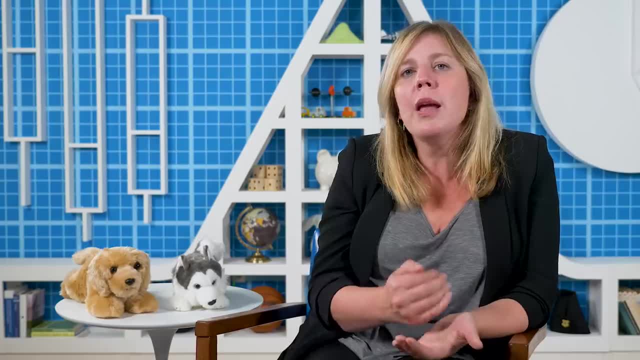 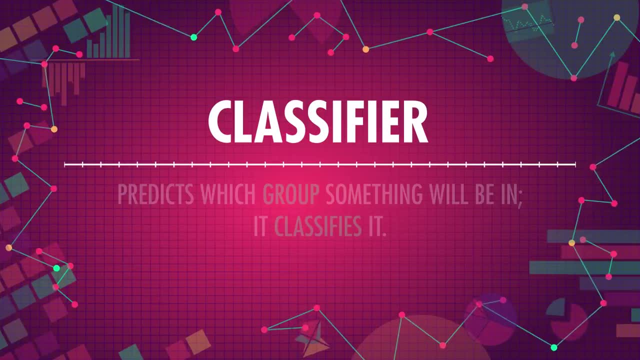 I'm going to take 20% of the data and just ignore it for now. Then I'm going to take the other 80% of the data and use it to train a k-n-n classifier. A classifier basically just predicts which group something will be in. it classifies. 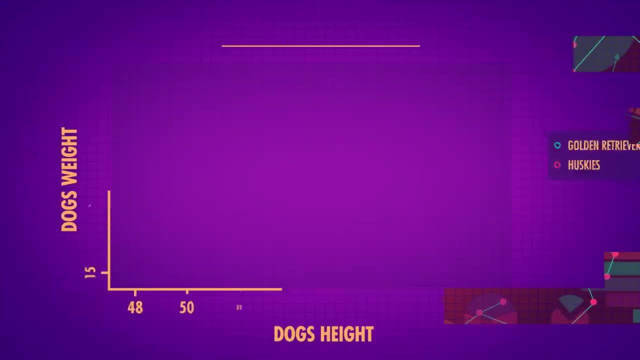 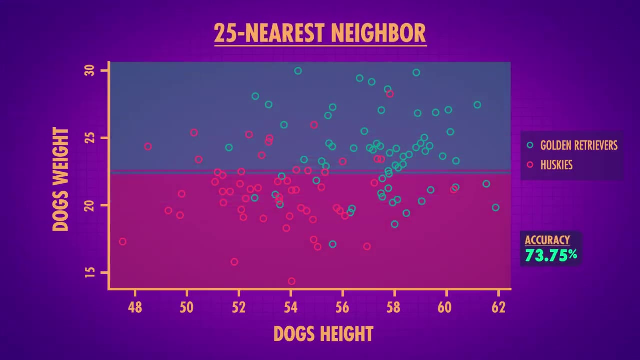 it, We'll build it And we get this result where blue means golden retriever and red means husky. As you can see, the boundaries between classes don't have to be one straight line. That's one benefit of k-n-n. 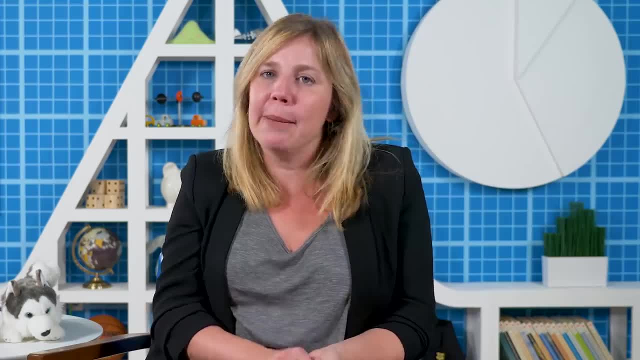 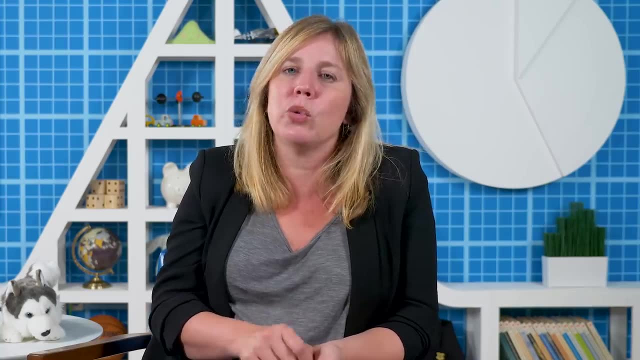 It can fit all kinds of data. Now that we've trained our classifier using 80% of the data, we can test it using the other 20%. We'll ask it to predict the classes of each of the data points in this 20% test set. 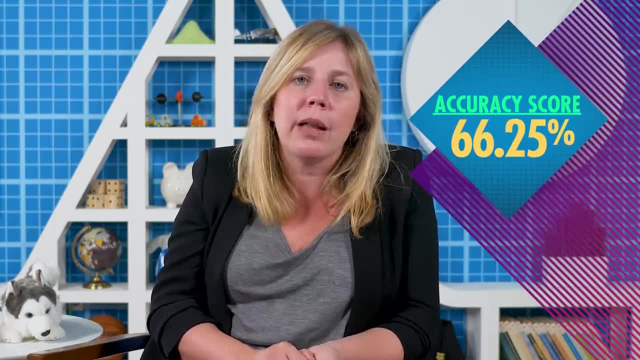 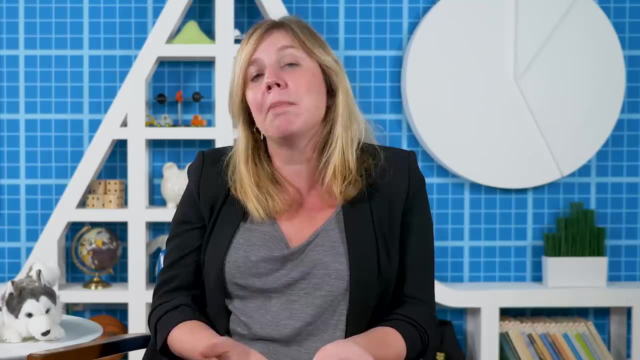 And again, we can calculate an accuracy score. This model has a 66.25% accuracy, So we can calculate the accuracy of each point, But we could also try out other k's and pick the one that has the best accuracy. 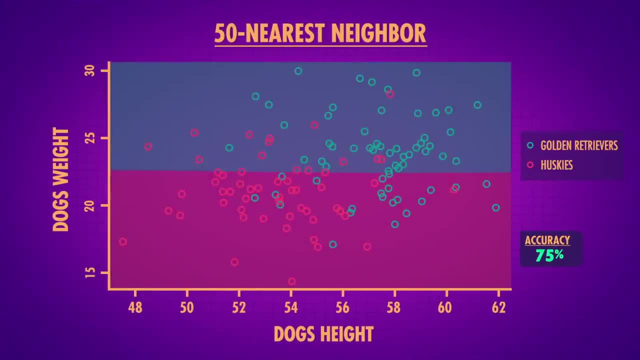 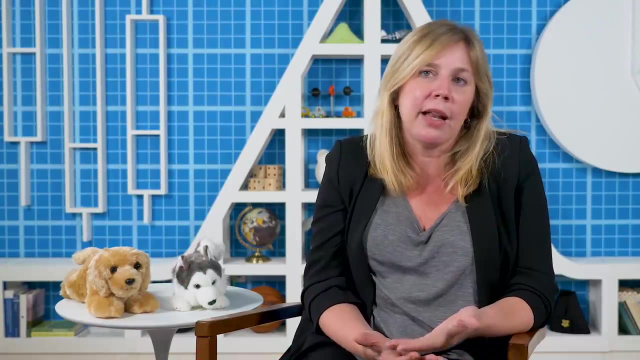 It looks like using a k of 50 hits the sweet spot for us, since the model with k equals 50 has the highest accuracy of predicting husky vs golden retriever. So if we want to build a k-n-n classifier to predict the breed of unknown dogs, we'd 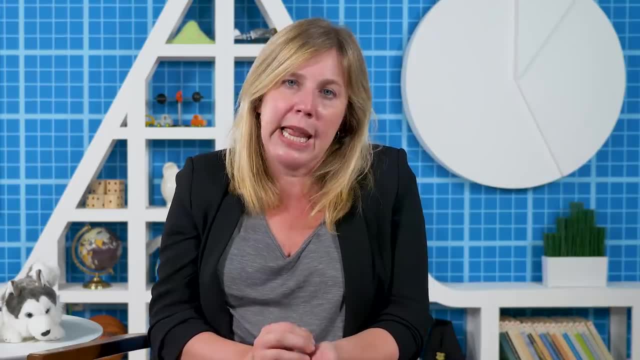 start with a k of 50.. Choosing model parameters, variables like k- that can be different numbers- can be done in much more complex ways than we showed here. Or it could be done using information about a dog, Or it could be done using information about a dog. 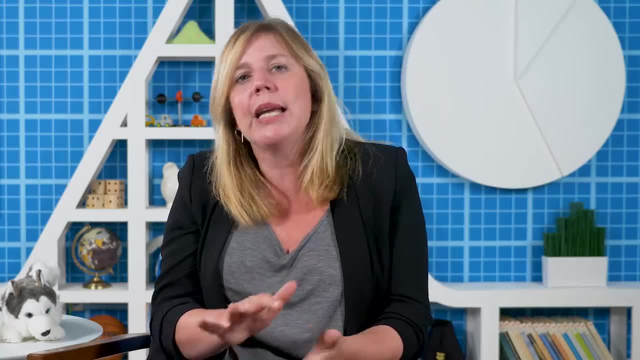 Or it could be done using information about a dog, Or it could be done using information about the specific data set you're working with. We're not going to get into alternative methods now, But if you're ever going to build these models for real, you should look it up. 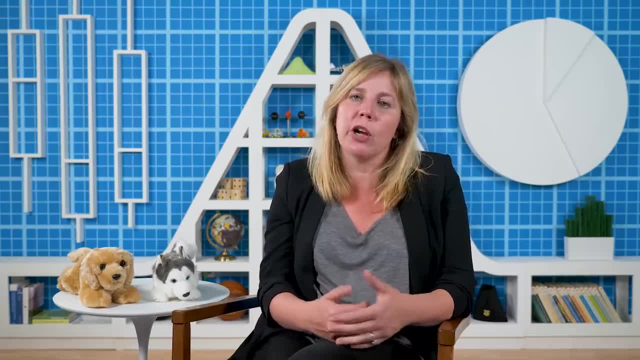 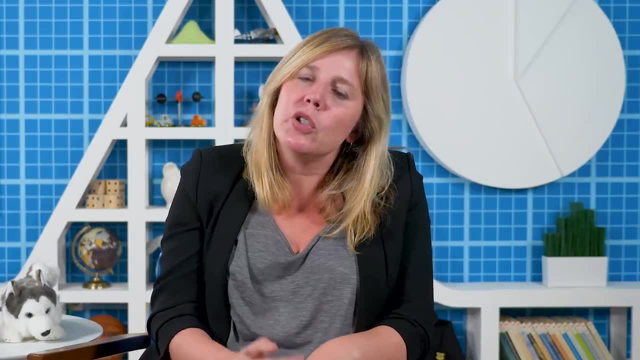 Machine learning focuses a lot on prediction. Instead of just accurately describing our current data, we want it to pretty accurately predict future data, And these days data is big. By one estimate, we produce 2.5 quintillion bytes of data per day. 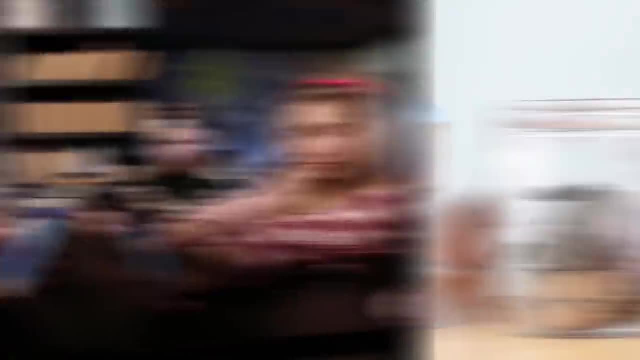 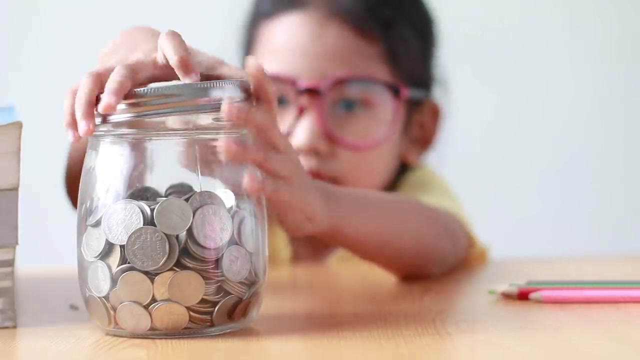 And supervised machine learning can help us harness the strength of that data. We can teach models, or rather have the models teach themselves, how to best distinguish between groups that will pay off a loan and those that won't, Or people who will watch the new season of The Good Place and those that won't. 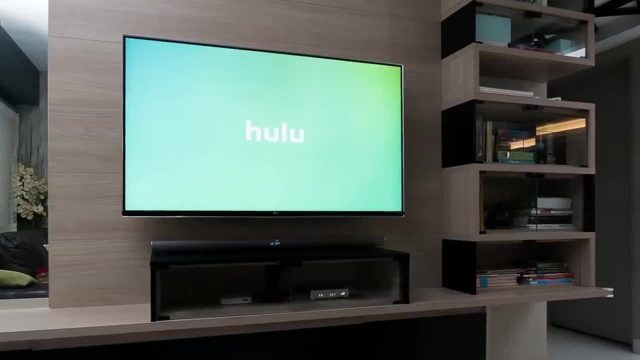 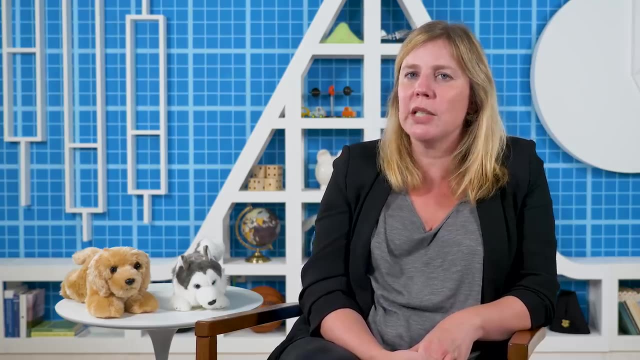 We're affected by these models all the time, from online shopping to streaming a new show on Hulu to a new song recommendation from Spotify. But machine learning doesn't always make it better. We're gonna get to that. Thanks for watching. I'll see you next time.